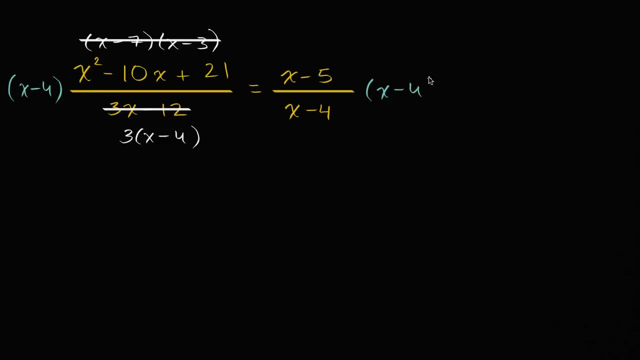 x minus 4, and then x minus 4,. that and that cancels, that and that cancels, and then we're left with, in the numerator, we're left with our x squared minus 10x plus 21,, and let's see: divided by 3, divided by 3 is equal to x minus 5.. 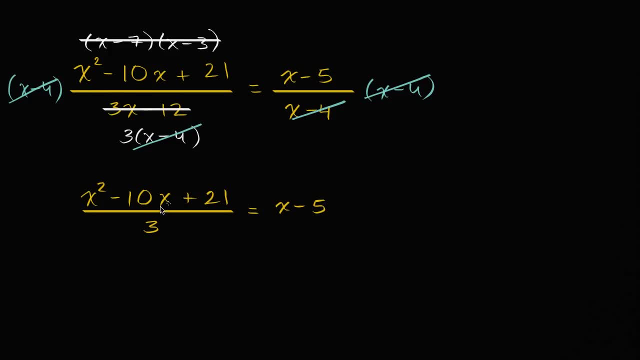 Let's see now what we could do- and actually I could have done it in. the last step is I could multiply both sides by 3, multiply both sides. do that in another color, just so it sticks out a little bit more. 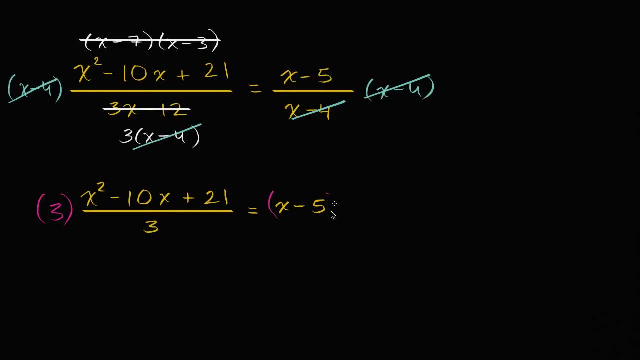 So I can multiply both sides by 3,, so multiply both sides by 3.. On the left-hand side, that and that cancels, and I'll just be left with x squared minus 10x plus 21, and on, and I don't have a denominator anymore. my denominator is 1, so I don't need to write it. 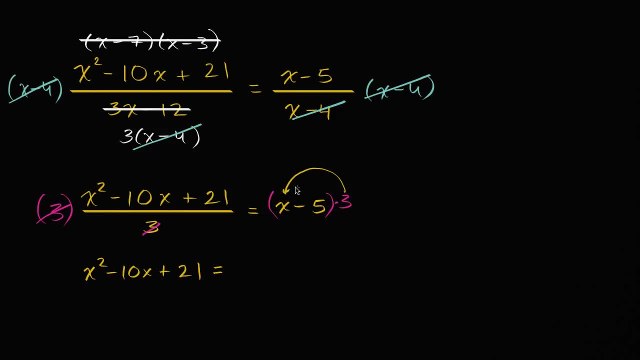 is going to be equal to 3 times. let's distribute the 3, 3 times x is 3x. 3 times negative. 5 is negative 15.. And now I can get this in the standard quadratic form by getting all of these terms onto the left-hand side. 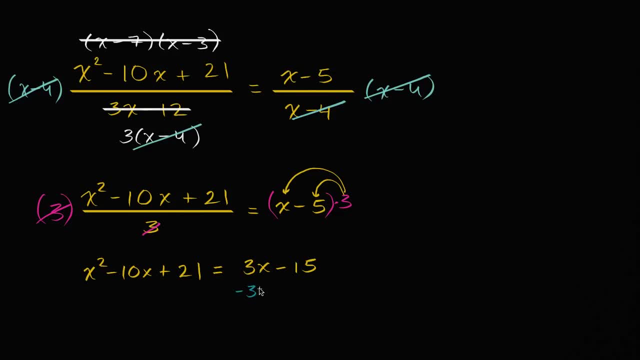 The best way to do that. let's subtract 3x from the right. but I can't just do it from the right, otherwise the equality won't hold. I have to do it from both sides if I want the equality to hold. 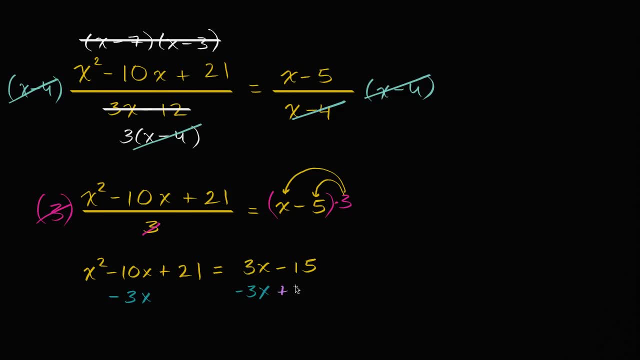 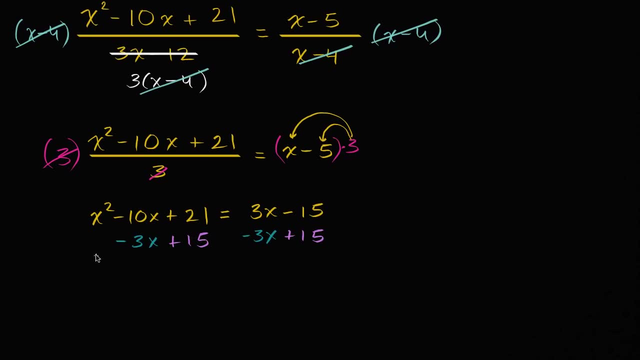 And I want to get rid of this negative 15, so I can add 15 to both sides. So let's do that, and what we are left with scroll down a little bit so I have a little more space. what we are going to be left with is x squared minus 13x. 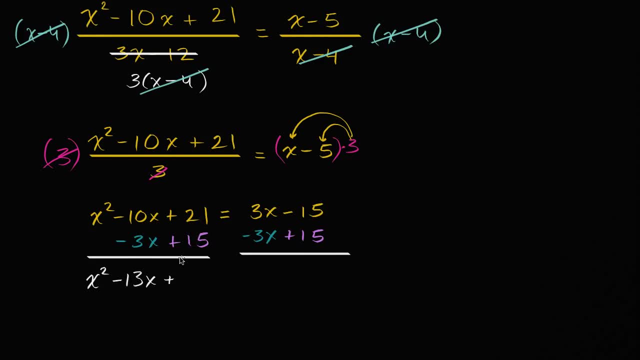 and then plus what is this? plus 36,, plus 36,. did I do that right? Yeah, plus 36, is equal to is equal to 0.. Alright, now let's see. we have this quadratic in the standard form. how can we solve this? 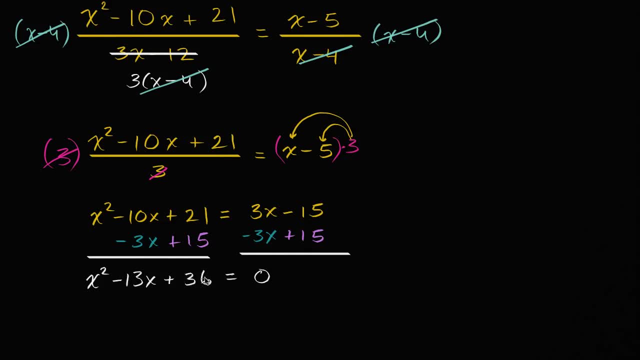 So, first thing, can we factor this Product of two numbers, 36,. if I add them, I get negative 13,. they are both going to be negative, since they have to have the same sign to get their product to be positive. And let's see 9 and 4 seem to do the trick. 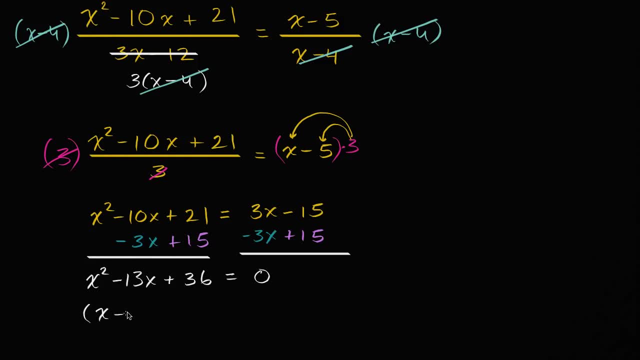 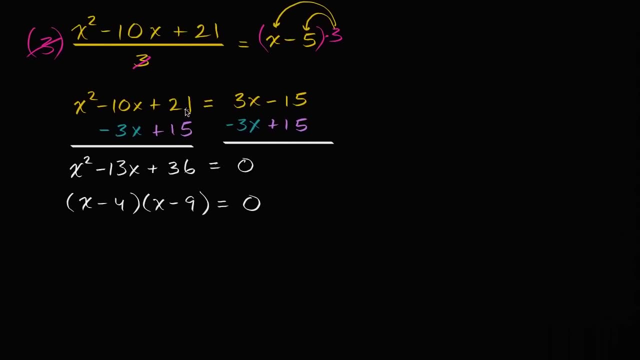 so or negative 9 and negative 4,. so x minus 4 times x minus 9 is equal to 0,. well, that's going to happen if either if either x minus 4 is equal to 0, or x minus 9 is equal to 0,. 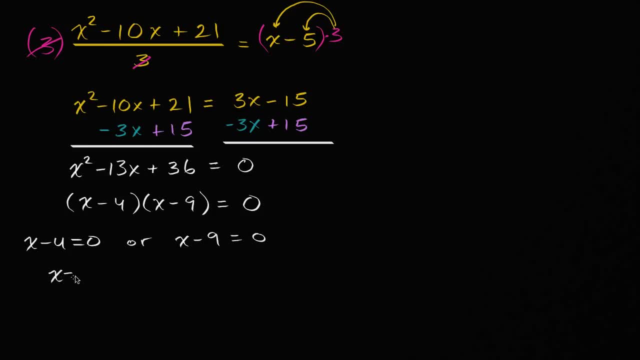 well, add 4 to both sides of this. this happens when x is equal to 4, add 9 to both sides of this. this happens when x is equal to 9.. So we could say that the solutions are x equals 4 or x equals 9,. 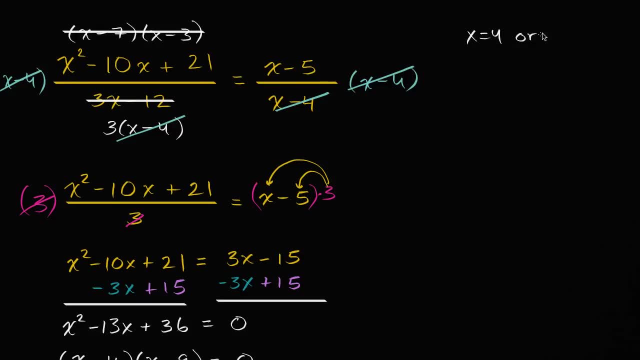 so x is equal to 4, or x equals 9,. but we need to be careful because we have to remember, in our original expression x minus 4 was a factor of both denominators and so if we actually tried to test x minus 4 in the original equation, 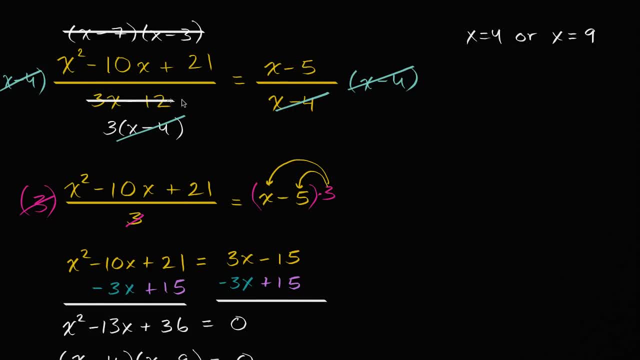 not one of these intermediary steps in the original equation I would end up dividing by 0 right over here and actually I would end up dividing by 0 right over there as well. So the original equations. if I tried to substitute 4,. 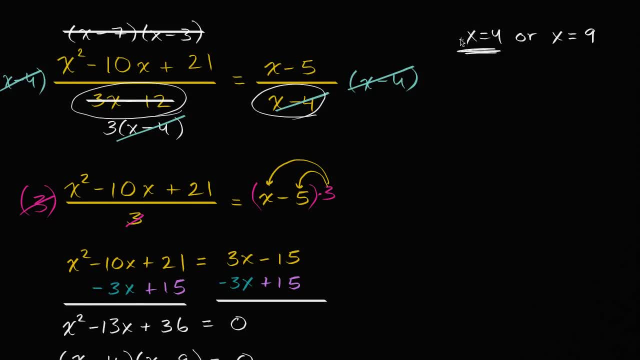 they don't make sense. So this is actually an extraneous solution. it's not going to be a solution to the original equation. the only solution is: x is equal to 9.. 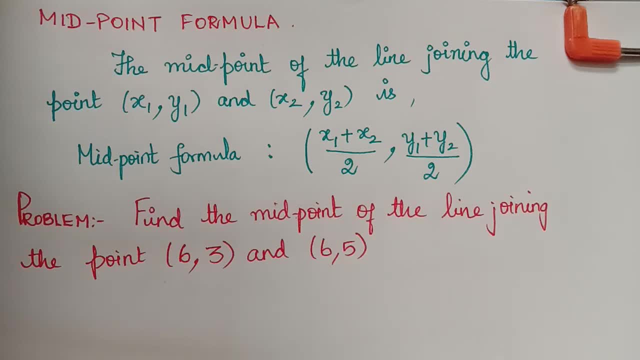 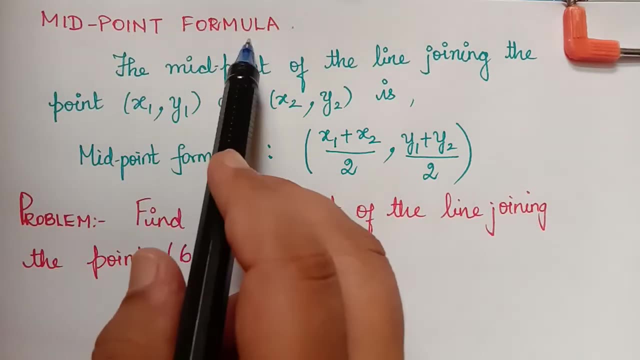 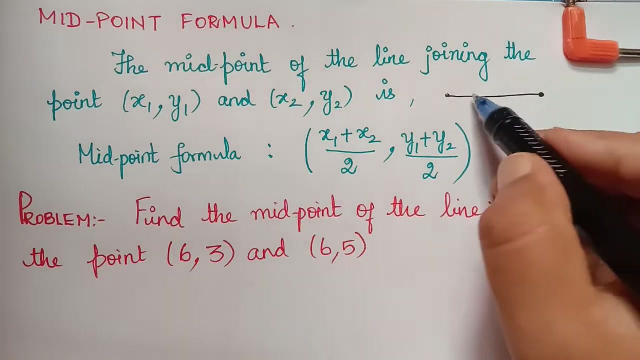 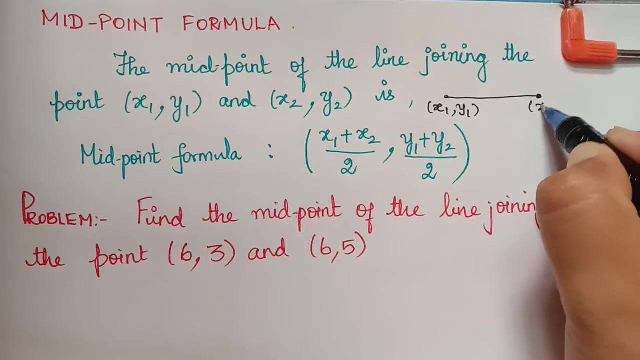 Hello students, the next formula under the topic coordinate geometry that we are going to learn is midpoint formula. So now, first we should know what is a midpoint. So in a line segment, we know that a line segment joins two points and if suppose the points are x1, y1 and x2, y2,.